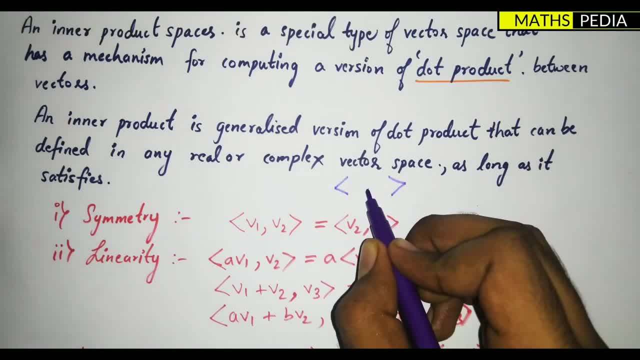 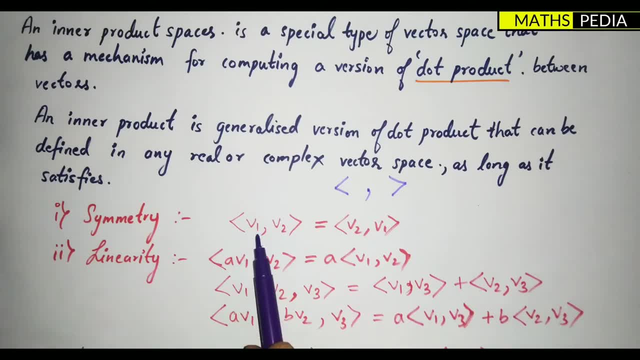 sign that symbols: okay, and in between the vectors we will put one comma. okay. So that is given. here we will say it as inner product of v1 and v2 vectors. Now that is equal to what? inner product of v2 and v1.. Here it is nothing but symmetry, the opposite of this, or we can say conjugate of: 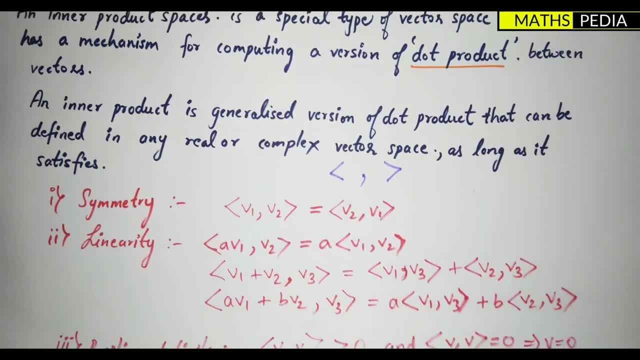 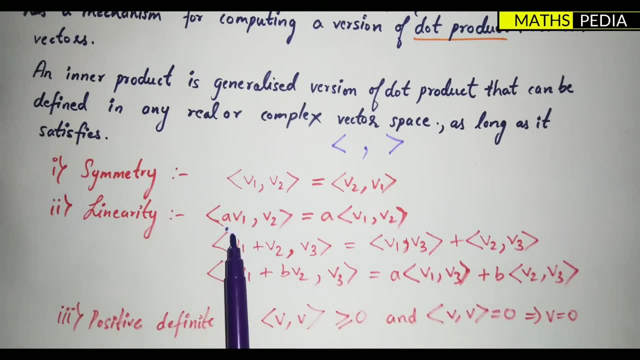 the vectors. Now, this is the first property, or the condition. Second one is the linearity property where, in case we have a which is nothing but the scalars, okay, scalar and v1, v2 are the vectors. The linearity property is v1 plus v2 and v2 is equal to. we will take what scalar outside and inner. 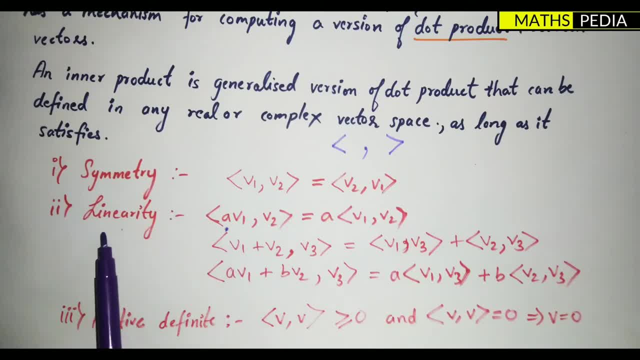 product of v1 and v2. that is it okay. The second one is that by in the under the linearity property itself, v1 plus v2, inner product of v1 plus v2 and v3. these three are what vectors and what we will. 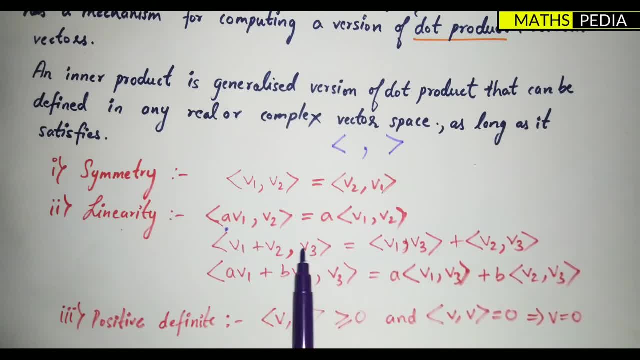 get. we will get it as v1- v3, inner product of v1, v3 plus v2- v3.. So it is nothing but the scalar outside. that is it okay? Now the third one is a- v1 plus b- v2, where a and b are the scalar and that we should. 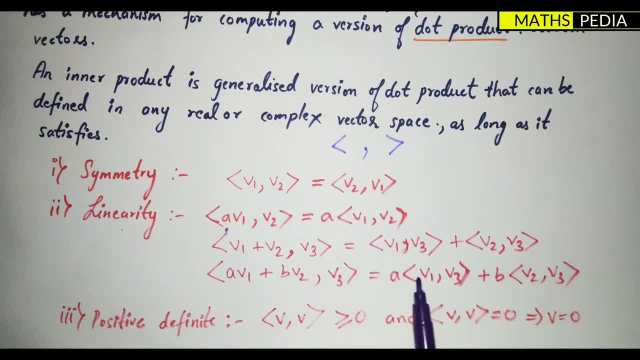 take it outside. So basically we are taking a outside and inner product of v1 and v3. it is same as this thing, just I have added here scalars a and b. that is it okay? So we have to just take a outside and here also b outside, rest all is same as the second one And the third and the 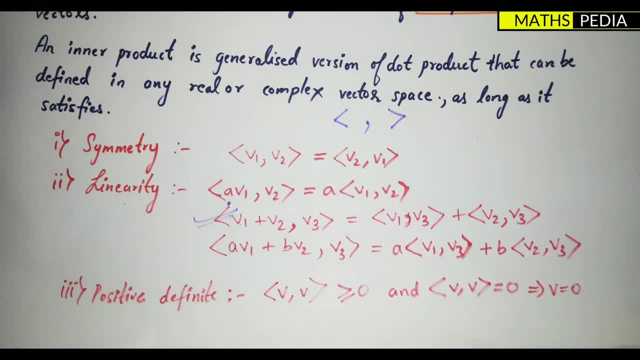 last condition is that positive definite property it is nothing. but if you are considering a vector, v, whose inner product we are taking v, inner product of v and v- these both are the same vectors- it will be greater than or equal to zero. this point you have to remember, okay. So whenever 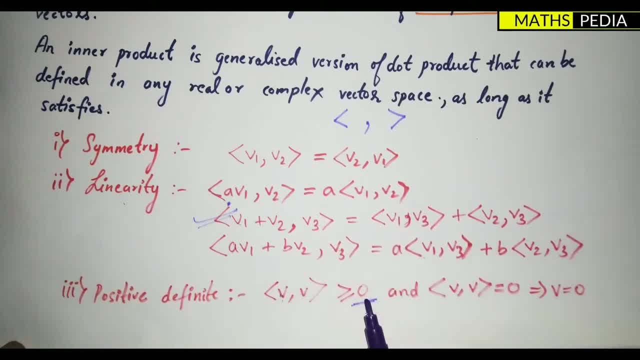 we calculate the inner product of the same vector, then we it should be what greater than or equal to zero. If it is equal to zero, then we should. that implies what Vector will be what Zero? That will say when we solve some certain problems based on this. okay. 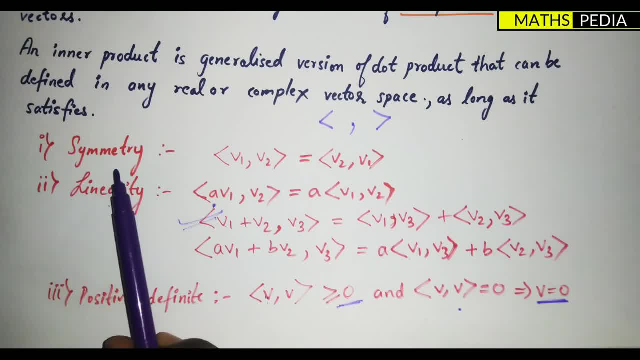 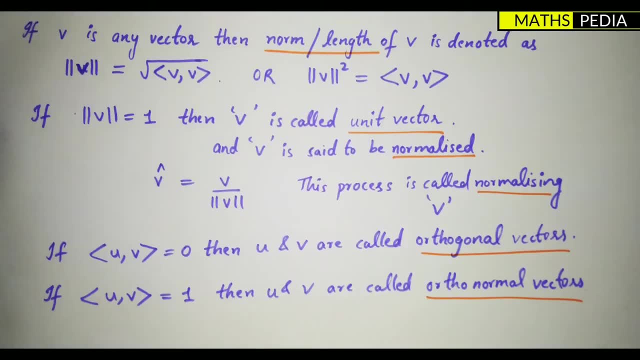 So you have to understand these three condition. the first one is symmetry- we call it as conjugate also- then linearity, then positive definite property. Now we will see some more few important points based on the inner product spaces. okay, Before solving some problems we have to see, look. 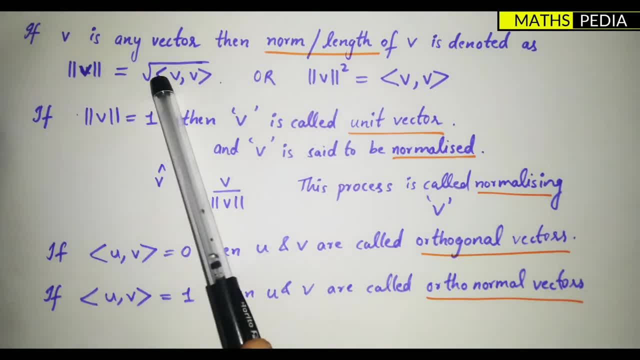 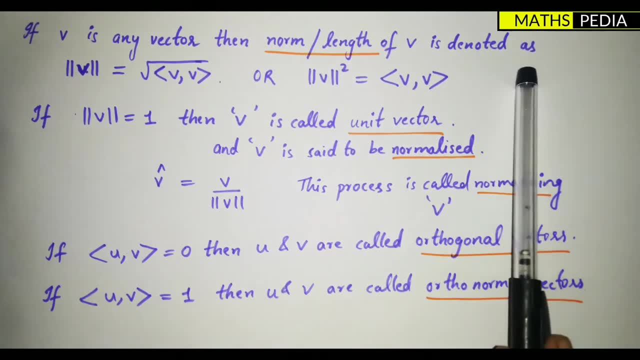 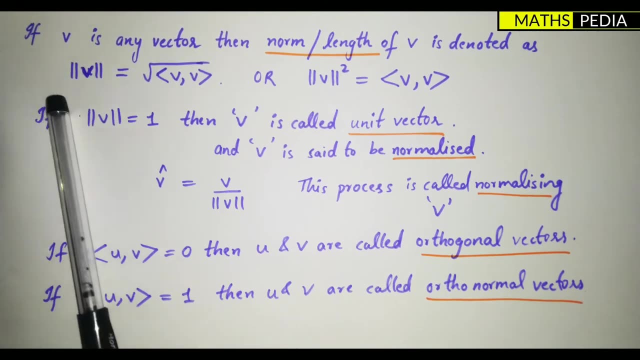 into some important points. The first one is: if v is any vector, then norm or length, We call it as norm or length of v vector it is denoted by. this is the important point. If we are to calculate the norm or length of the vector, we have to use this symbol. this is nothing but the 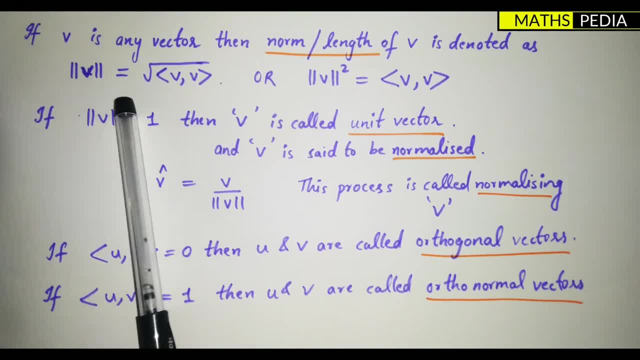 symbol of norm or a length of a vector. It is given as under root of inner product of the same vectors. okay, You can observe here v. I have taken the vector. here it is nothing but double line straight lines. I have given here vertical lines. this is the we can say notation of norm. 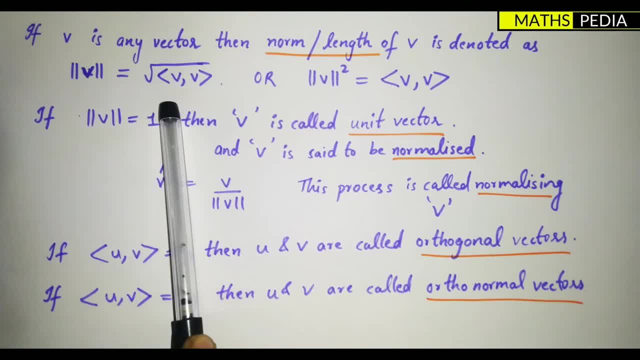 Or length, and how to calculate it is nothing but under root of square, root of inner product of the same vectors. okay, which should be equal, greater than or equal to this property we have discussed, or in other words we can say the norm of a length of vector v, square, square of that, it is equal to. 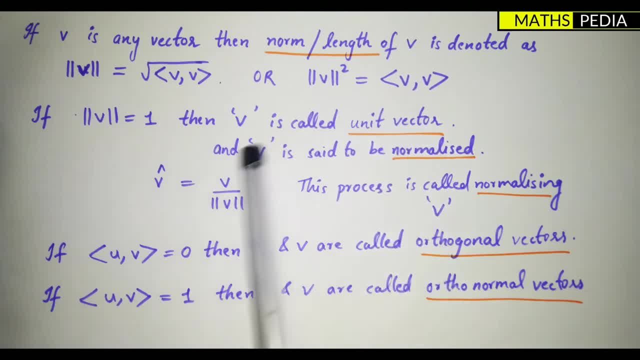 what in a product of the same vectors. Now the second point. if the norm of vector v, if it is, then v is called as what unit vector and v is said to be normalized when, if v norm of v is equal to what one, Next one is, if we are supposed to suppose we will take one unit vector, this is the unit. 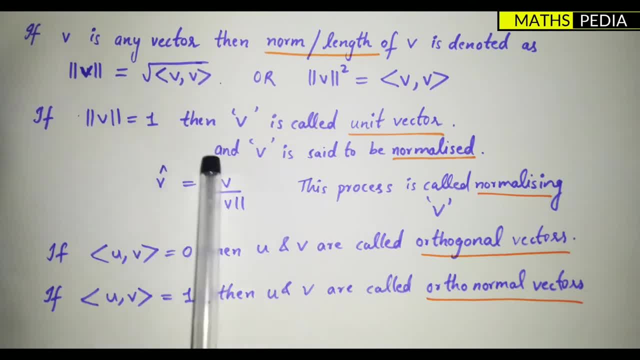 vector. if v is any vector, okay, then the unit vector is denoted by what vector, by norm of that vector, norm or length of that vector, and this process is called as unit vector. So if we are finding out the unit vector, this is called as what? normalizing vector v. okay, this is nothing but. 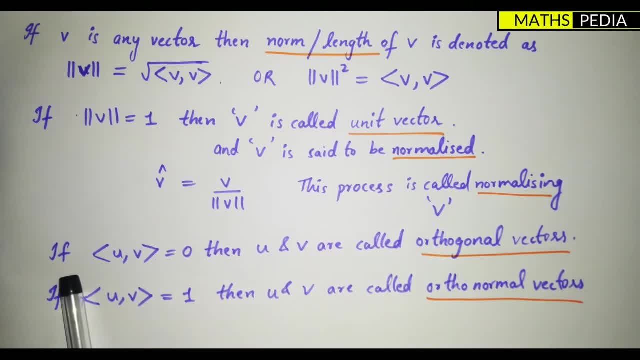 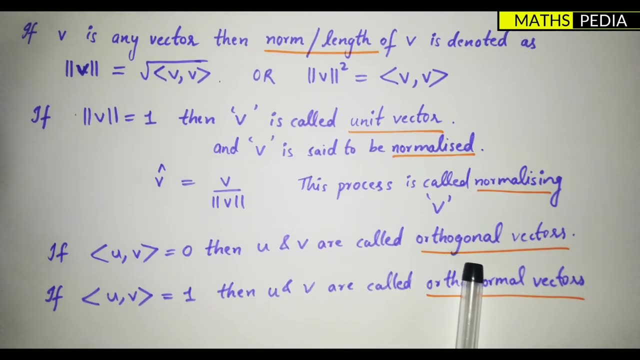 normalizing. Now the next point is: if suppose if unit or inner product of u and v vector, u and v be any vectors, okay, so if it is equal to 0, then u and v are called orthogonal vectors. This point is important. orthogonal vectors and orthonormal vectors. Orthonormal is not a vector vector. 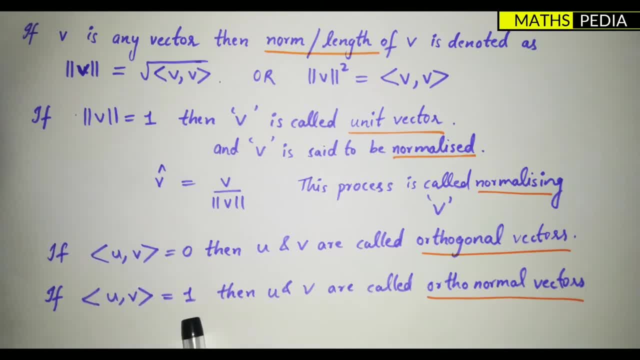 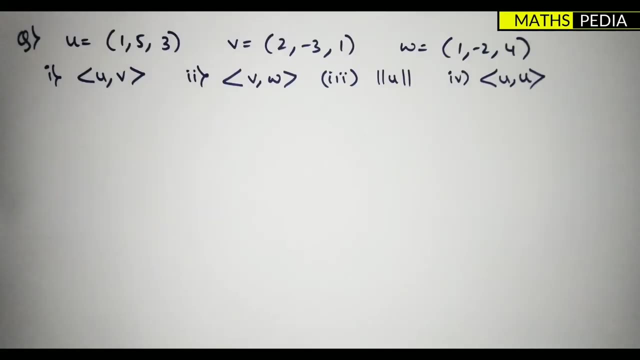 but when the inner product of u and v vectors are is equal to what 1? okay, so this, after discussing this, all properties or and the important points, let us go with the solving some problems, Guys. let us solve the problems based on this inner product. Now, u vector is given v vector. 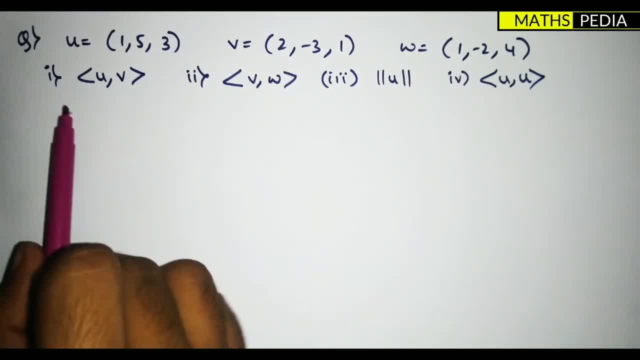 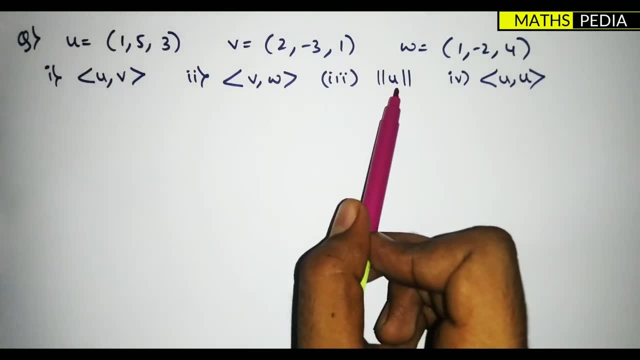 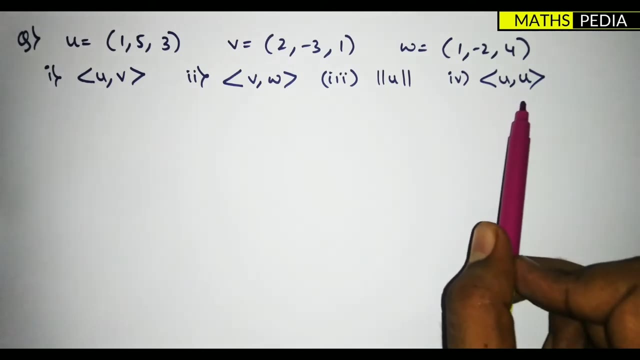 is given and w vectors are given. okay, those three vectors are given. Now they are asked to find out of: between u and v, v and w and norm, or we can say length of the u vector and even the u vector inner product of u vector. that means the same vectors. okay, so let us take with the first one. 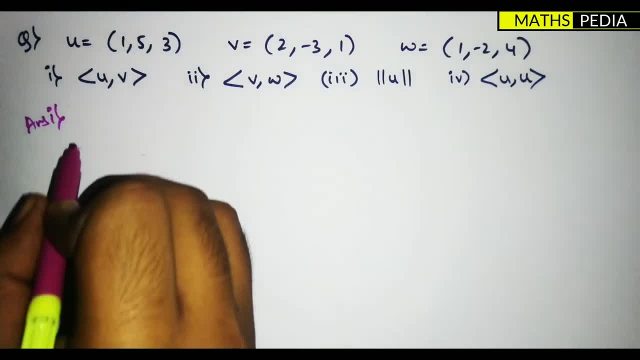 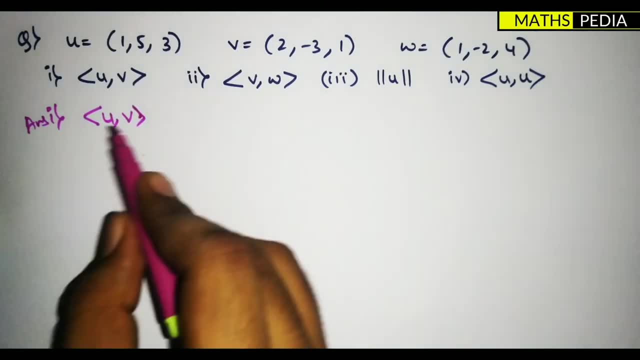 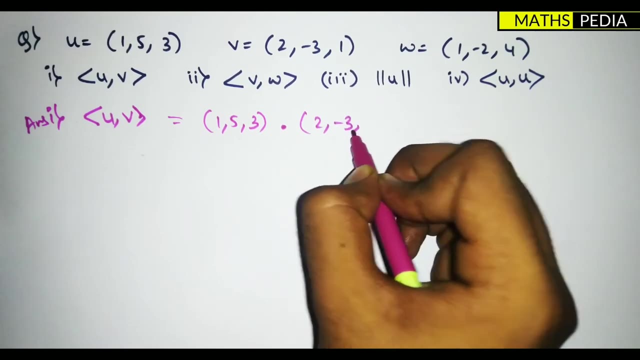 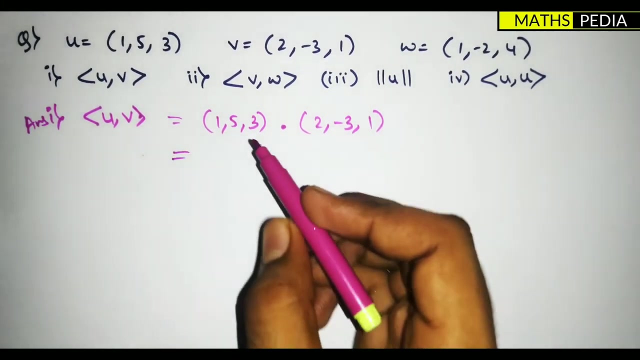 so for solving the first one, inner product means what we have to find the dot product between the vectors. so basically, first i'll write the vectors. so 1, 5, 3 dot product with 2 minus 3, 1. i've just wrote the u and v vector dot product of both of them. now, in order to do 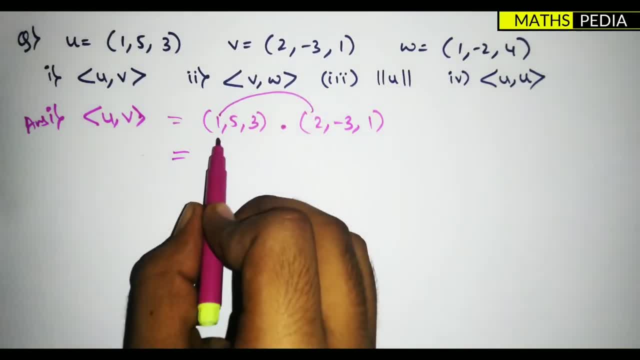 the dot product. you have to just multiply with the respective this we can say x, y, z and z coordinates, and just you have to multiply. you have to just multiply with the respective this we can say x, y, z and z coordinates, and just you have to multiply. 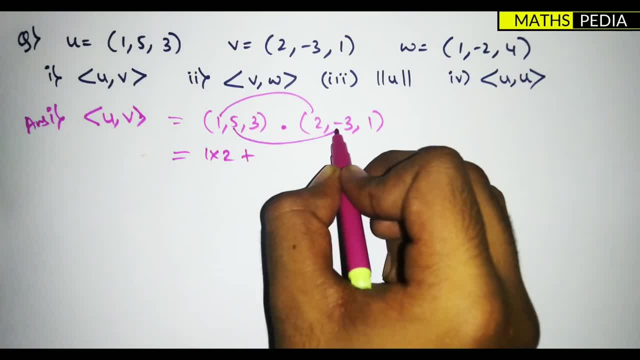 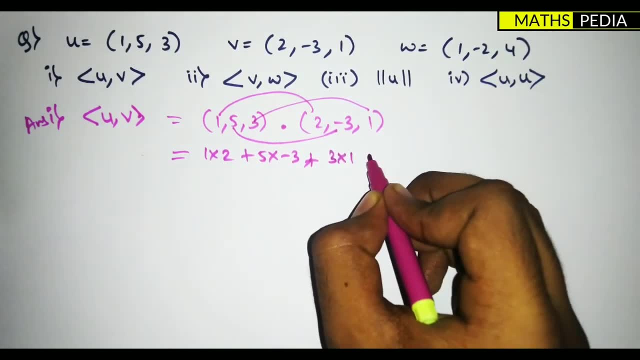 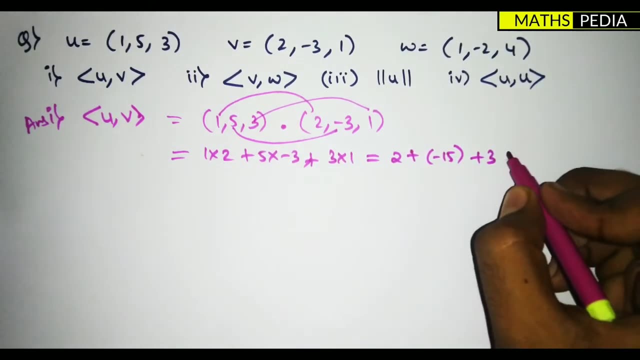 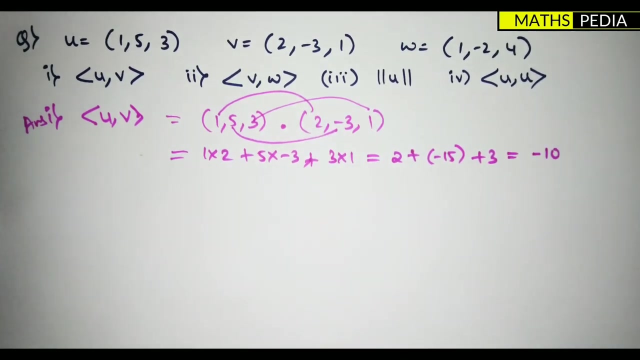 okay, so 1 into 2 plus 5 into minus 3 plus 3 into 1, so it is equal to 2 plus minus 15 plus 3, which is equal to what minus 10? so let us do the second question now to find the inner product of v and. 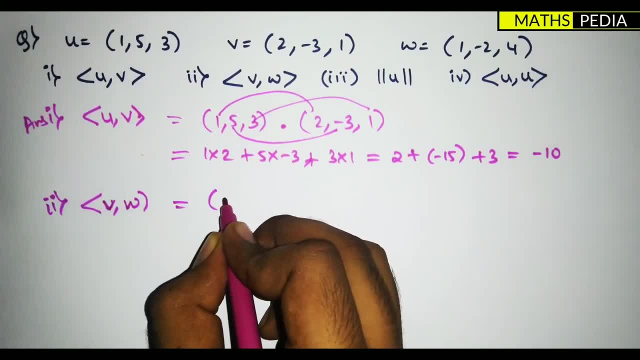 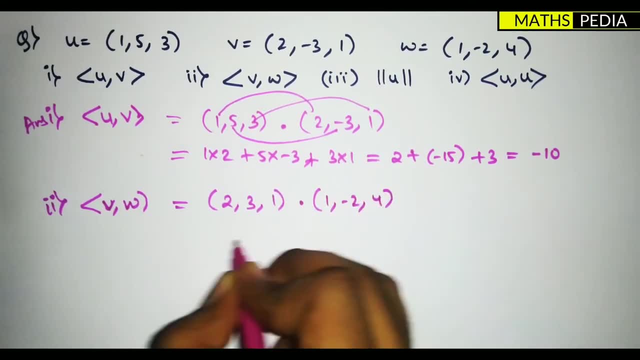 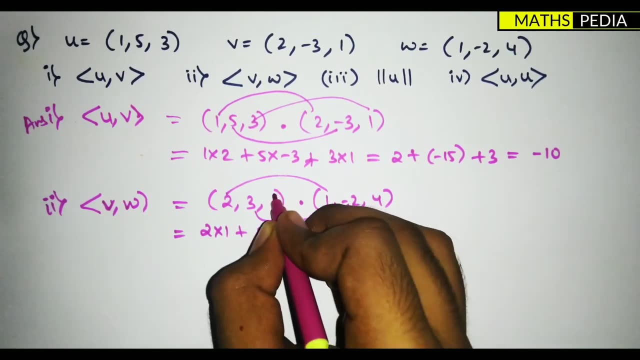 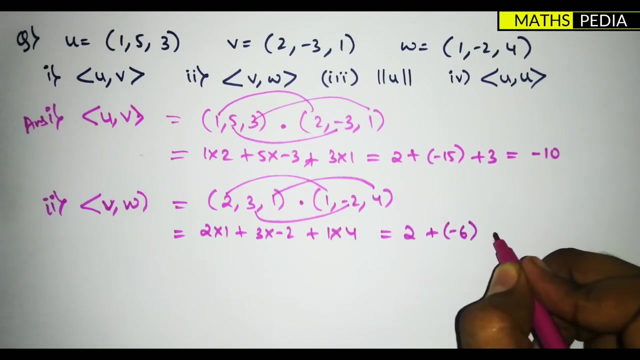 w. so first i'll write v, vector 2, 3, 1, so 2 into 1 plus 3, into minus 2 plus 1 into 4, which is equal to 2 plus minus 6 plus 4, so which is equal to equal to what. 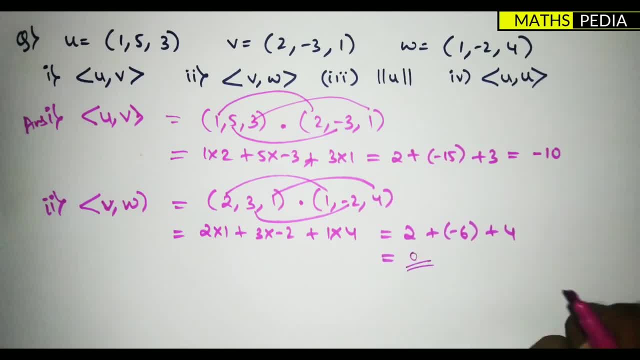 6 plus 6 minus 6, it is equal to 0. so this is one example of what orthogonal vector. okay, this is example of what orthogonal vector where that means these two vectors which one, v and w, are nothing but the orthogonal vectors, since the inner product of these two, we got it as what? 0. okay, if suppose. 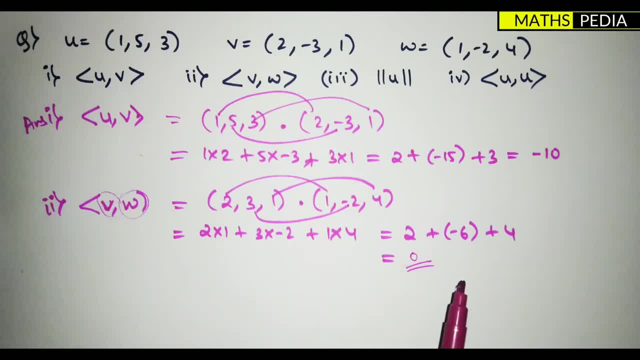 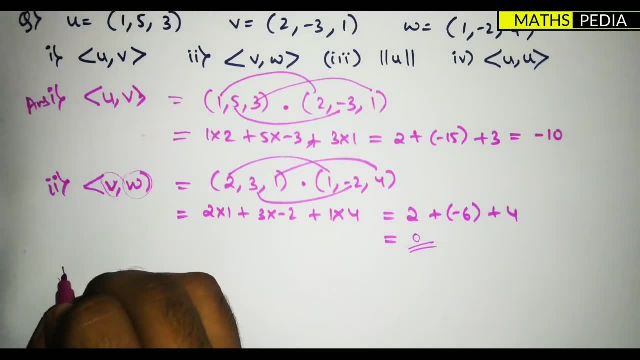 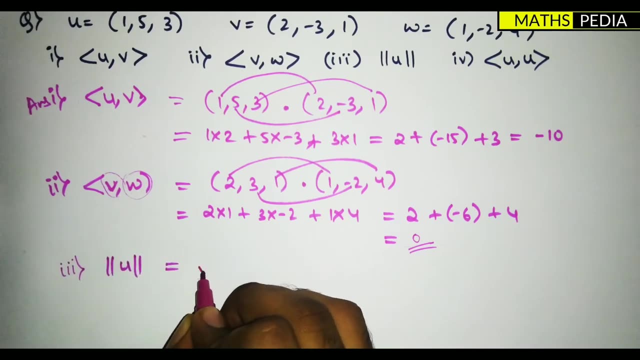 the inner product of these two vectors are equal to is equal to what? 1. then it is orthonormal vectors. okay, so let us do the third one. third one is nothing, but we have to find the norm. so we have the formula for that. how to find the norm which is equal to what under root of inner. 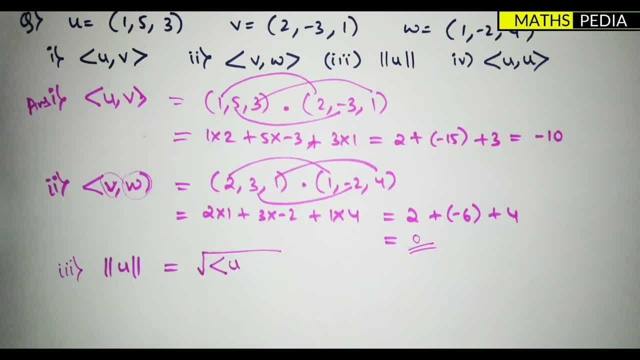 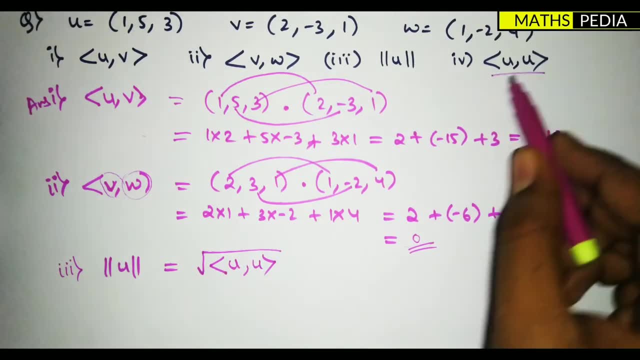 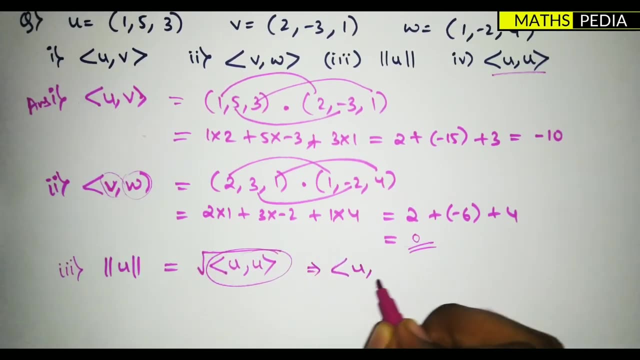 product of u comma u. okay, so it is nothing but this we are finding out. it is nothing but the fourth answer itself. so let us do first this one, so we'll find out first the inner product of the u vectors. now, that is equal to 1, 5 3. 1 5 3. 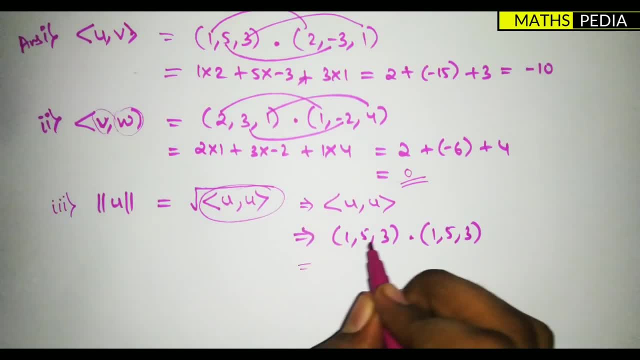 you have to just multiply 1 into 1 plus 5 into 5 plus 3 into 3, which is equal to 1 plus 25 plus 1 plus 25 plus 9, which is equal to what? 35? okay, so this is nothing but the fourth answer itself. now we have to do the under root of this. 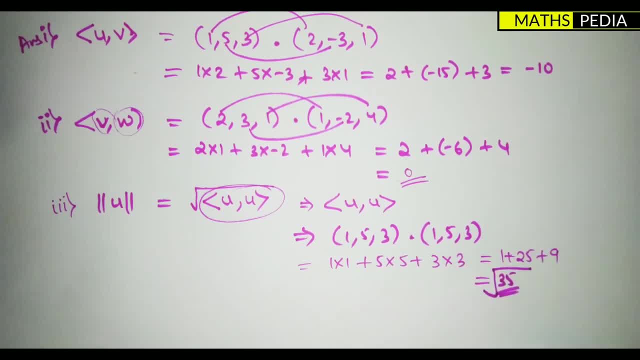 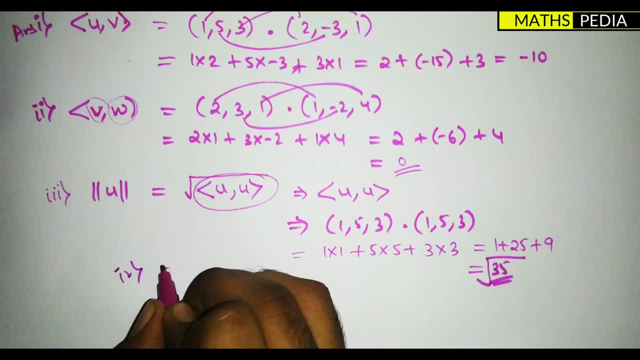 so just you do the square root of this. anyways, no need to calculate the square root, it is enough to write as square root of 35, okay, so fourth answer: we have it as what inner product of u and u vectors. it is equal to 35, okay. now the thing is that if you have observed that the 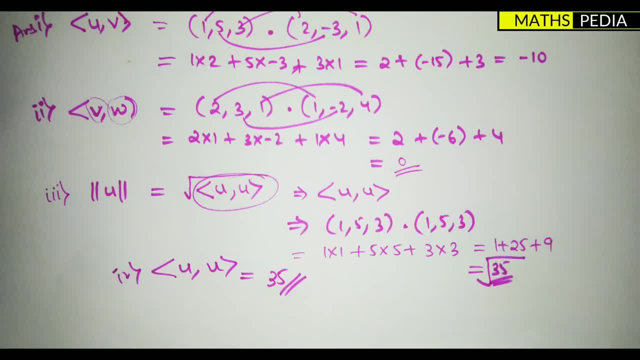 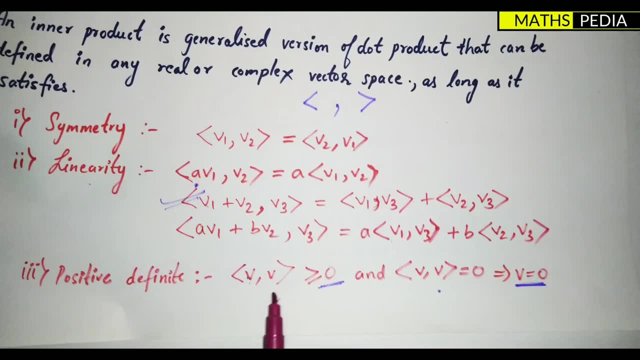 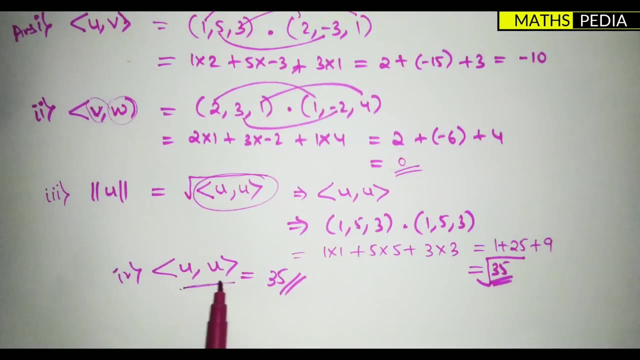 third property that we have discussed about: the positive definite. it is given over here. positive definite- inner products of the same vectors will be always greater than or equal to 0. okay, so that you can observe, here we have found out the inner product of the same vectors. you can try with the other vectors, taking up any of the examples.